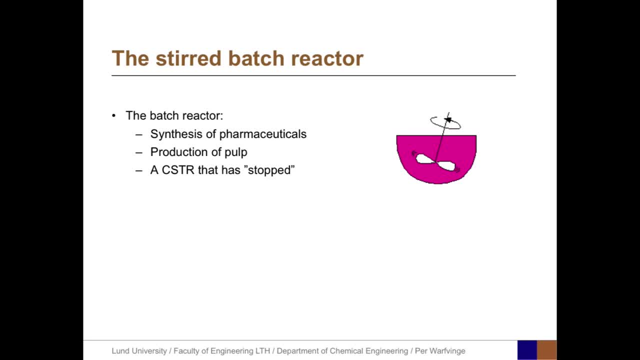 in a big batch in order to liberate the fibers that are used to make paper. A third example is when a CSTR has stopped, for example, when the pumps that provide the feed to the reactor have stopped, A batch reactor is closed- Closed with respect to matter and or with respect to energy. 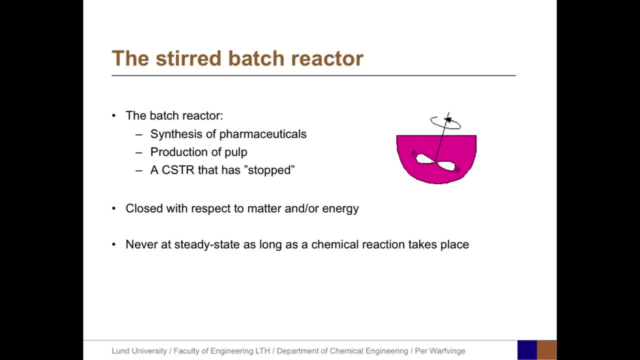 And the most important characteristic of the batch reactor is that it is never at steady state as long as a chemical reaction takes place within the reactor. Just as a CSTR, it is perfectly mixed. That means there are no gradients with respect to concentration or temperature within the reactor. 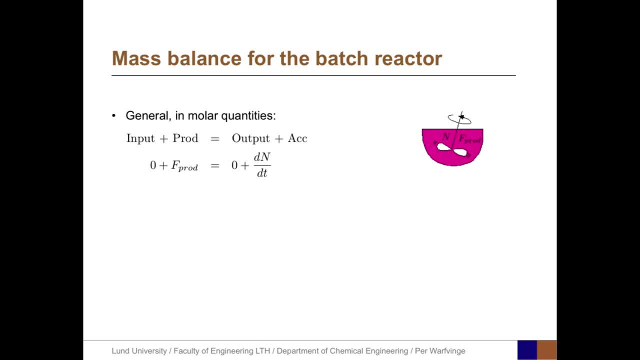 The mass balance equation for the batch reactor builds on the general mass balance equation. Input plus production equals the output plus the accumulation. However, since we do not have any input nor any output, we get F prod equals dN dt. That means that the molar rate of production from the chemical reaction 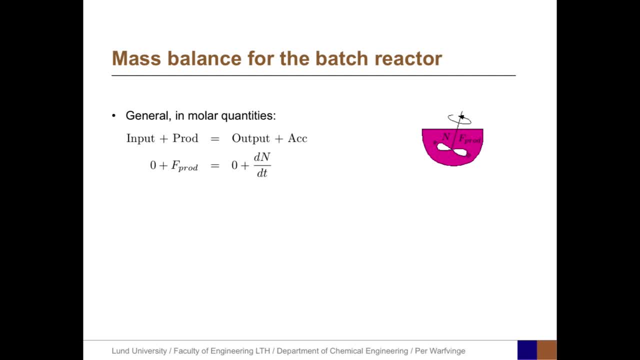 balances the change in molar amounts within the reactor. If we express this equation in preço quantities, we get: on the left side, r times v equals, and to the right side we have split the molar, r times v equals, and to the right side we have split the molar. 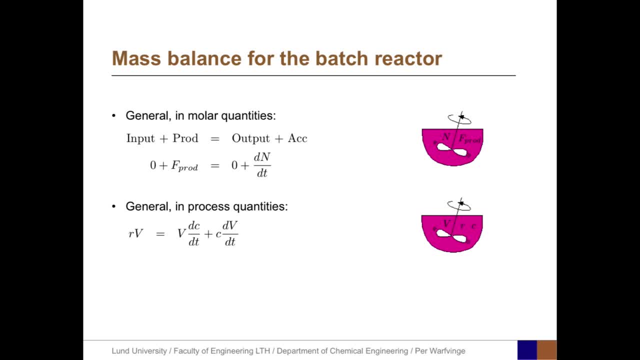 rate of change into two parts. The first part is V dC dt and the second part is C dV dt. If the volume is constant, the last term C dV dt, equals zero, And we then see that we can. 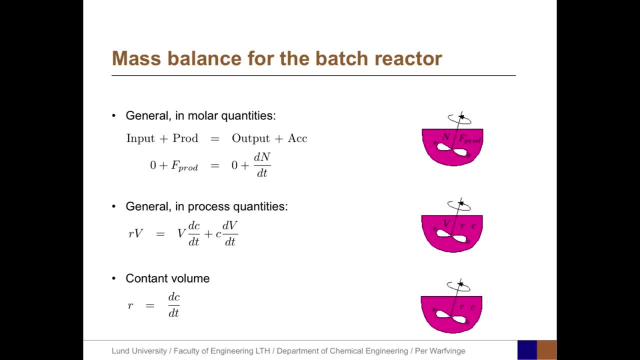 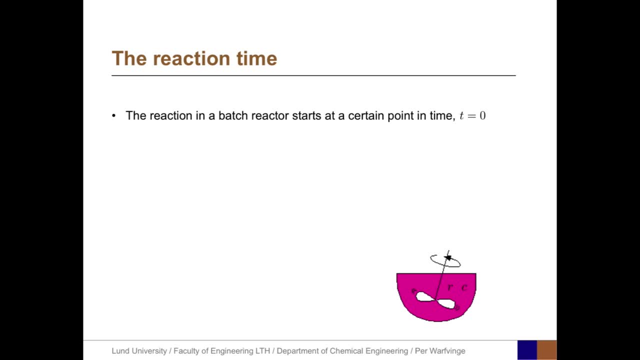 eliminate V both from the left side and from the right side to get the final equation: R equals dC, dt. The reaction time is different from the resonance time of a CSTR, since the reaction starts at a certain time when T equals zero, And at T equals zero, the concentration is the initial. 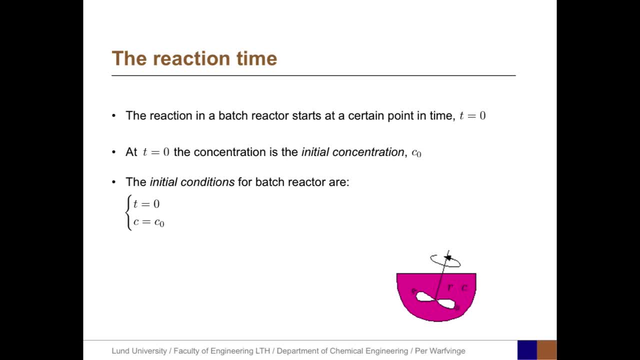 concentration. We call that C zero. The initial conditions for the batch reactors are at time equals zero. the concentration is the initial concentration And after a certain reaction time we have at any T greater than zero, the concentration Reactor. calculations for the batch reactor involve solving the differential equation: R equals dC- dt. 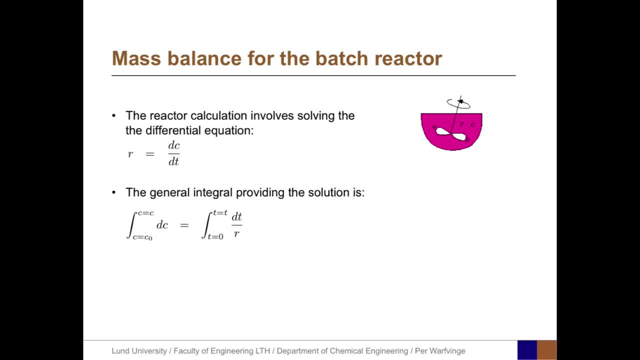 The general integral, providing the solution is: on the left side we integrate between the initial concentration and the final concentration, and to the right side we integrate between time equals zero and any other time. There are four steps involved in reactor calculations. The first step. 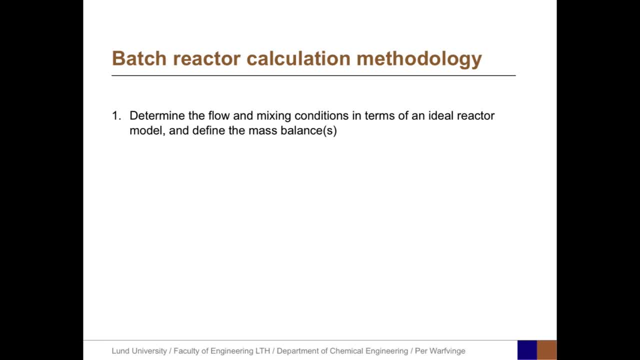 is to determine the flow and mixing conditions in terms of an ideal reaction. The second step is to define all the kinetic equations and the kinetic coefficients relevant for the system. The third step involves combining the mass balance equation with the kinetic equation to form the design equation. And the fourth step is to separate the variables and 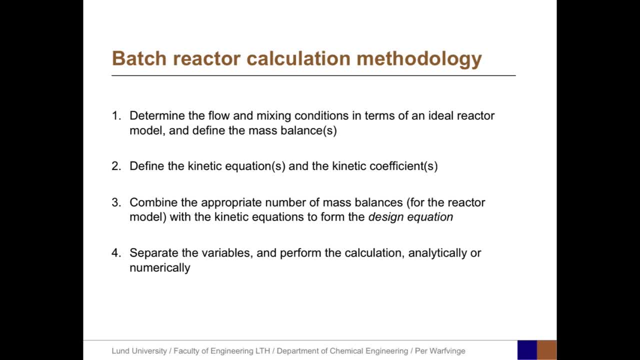 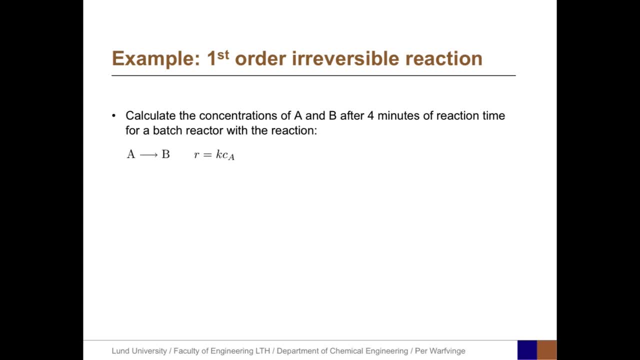 perform the calculation analytically or numerically. Let's turn to an example. Calculate the concentrations of A and B after four minutes of reaction time for a batch reactor. with the reaction A yields B and the rate equation is K times CA, The system properties are: 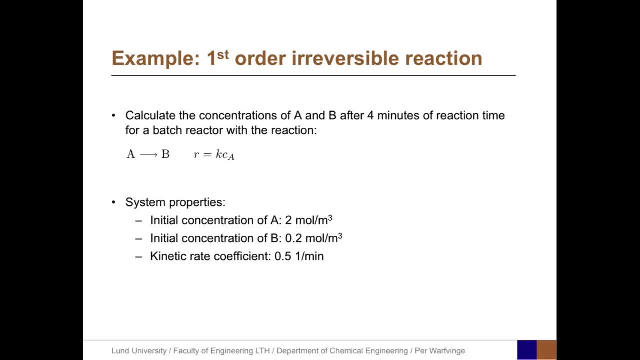 the initial concentration of A equals two moles per cubic meter, the initial concentration of B equals 0.2 moles per cubic meter and the kinetic rate equation for this first order reaction is 0.5 per minute. We have a batch reactor and the design equations that we need to solve are in order to calculate: 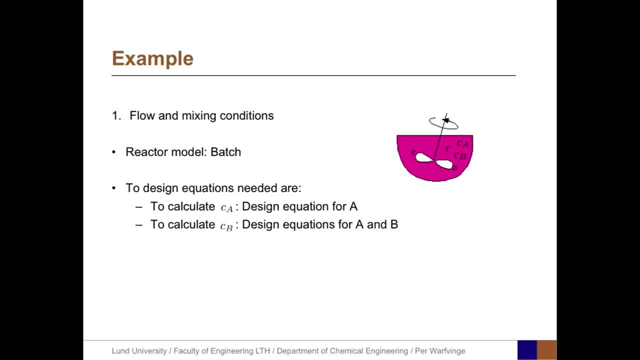 CA, we need to solve the design equation for A And to calculate CB, we need to solve both the design equation for A and the design equation for B. since CA is included in the kinetic equation that is used to calculate the formation of B, The mass balance equation becomes RA. equals to CA dt. 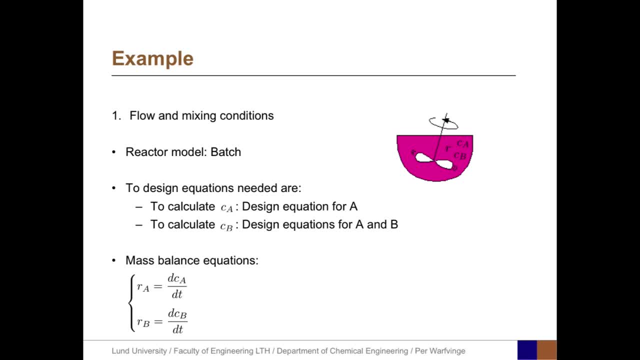 the mass balance equation for B is: Rb equals dCb, dT. The second step is to define the kinetic equations. This reaction is first ordered with respect to Ca. That means that the rate equation for the reaction is k times Ca. The rate equation 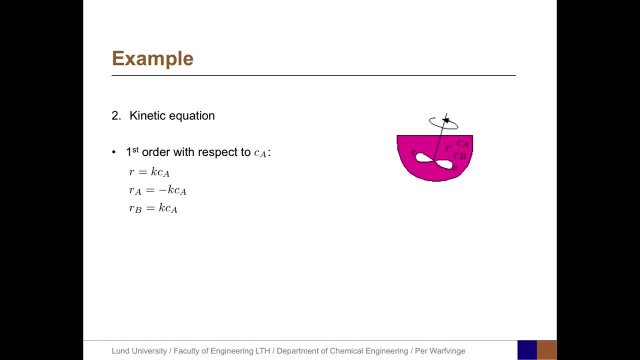 for the component A equals negative k times Ca, while the reaction rate for B, which is produced, equals k times Ca. The third step is to combine the mass balance equation with the kinetic equation to form the two design equations. The first one is negative kCa equals. 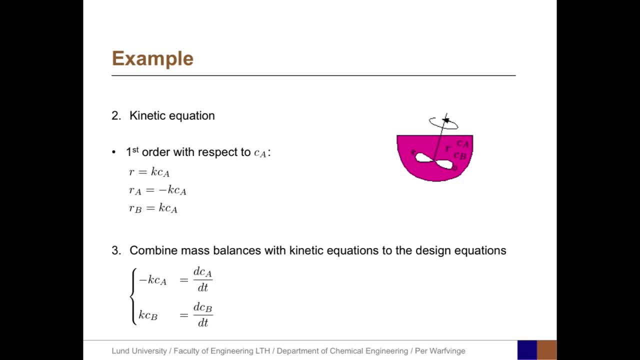 dCa- dT. while the design equation for B is k times Cb equals dCb- dT. We can now make the calculations and we have two strategies. Either we make a sequential equation where we first solve for Ca and then for Cb. 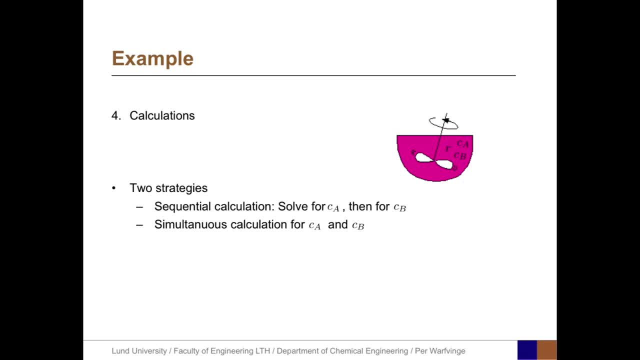 or we will make it simultaneously for Ca and Cb at the same time. Here we will apply the sequential calculation. The sequential strategy works for A, since the kinetic expression for the formation of A only includes Ca. On the first line we have the design equation turned the opposite way as on the previous. 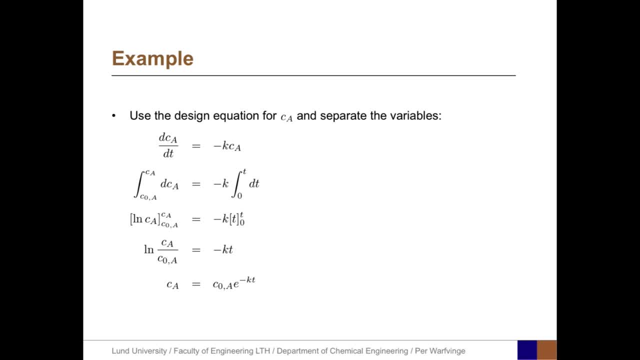 pages. In the second line the variables have been separated and the various boundaries have been included. The third line: we have the primitive functions with the various boundaries, and on the fourth line we have inserted the various boundaries on the left and the right side And on the 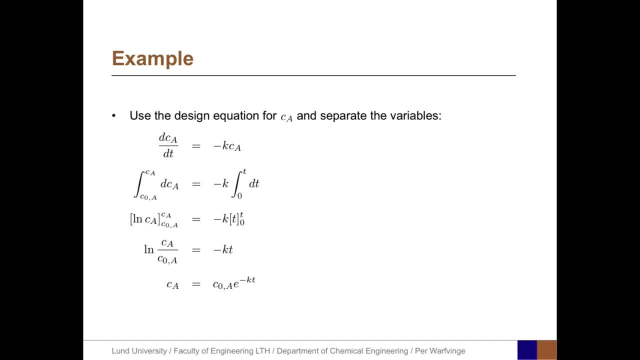 fifth line we have the final expression: Ca equals initial concentration of A times E to the minus k times T. With numerical values, Ca equals 2 times E to negative 0.5 times 4, and that is 0.278.. 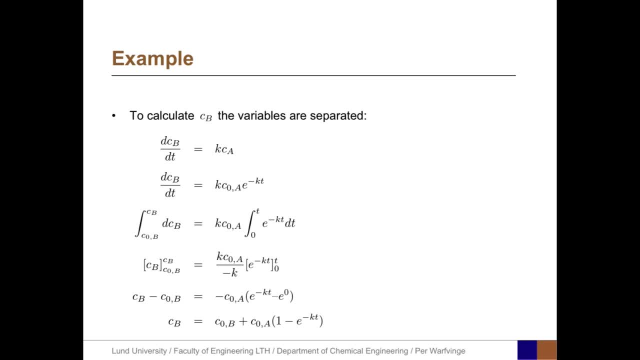 We can now calculate Cb. The first line: we have the design equation. On the second line, we have inserted the full expression for Ca into the right hand side of the equation. On the third line, the variables have been separated and the boundaries have been included. 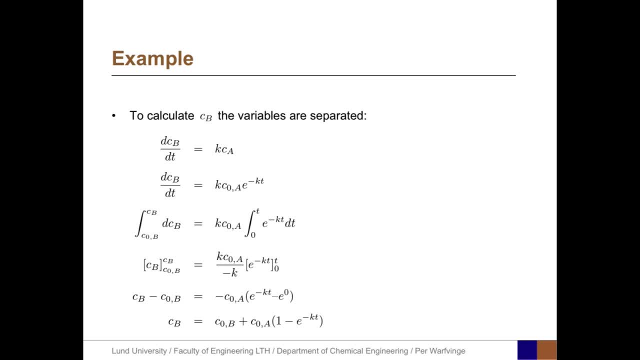 On the fourth line we have the primitive function and the boundaries. On the next line, this expression has been evaluated And on the last line we have the final expression: Cb equals the initial concentration of B plus the initial concentration of A times 1 minus. 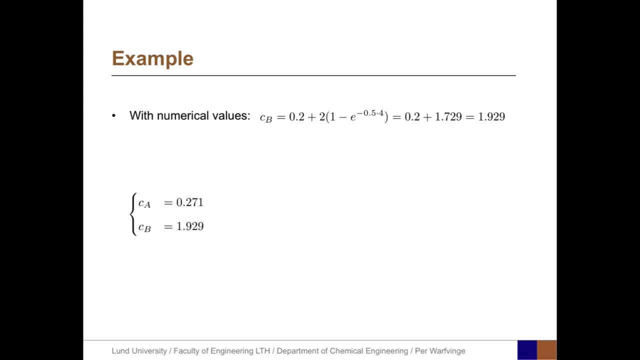 E to negative kT With numerical values. Cb is 1.929,, which means that after 4 minutes of reaction time, the concentrations are: Ca equals 0.271 and Cb equals 1.929.. If we add these concentrations, 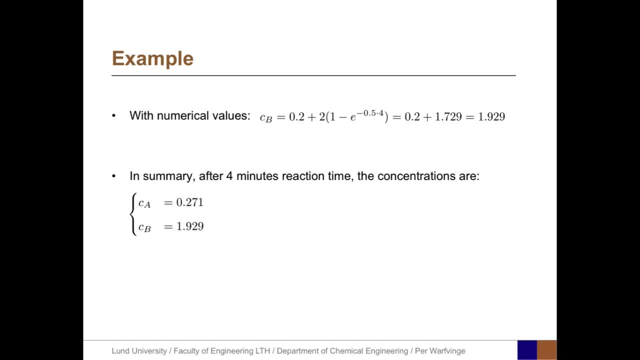 we get 2.2, which is logical, since that is also the sum of the initial concentrations and there was no change in total number of moles in the reaction. When we define conversion, we must define that in terms of molar amounts in the reactor.